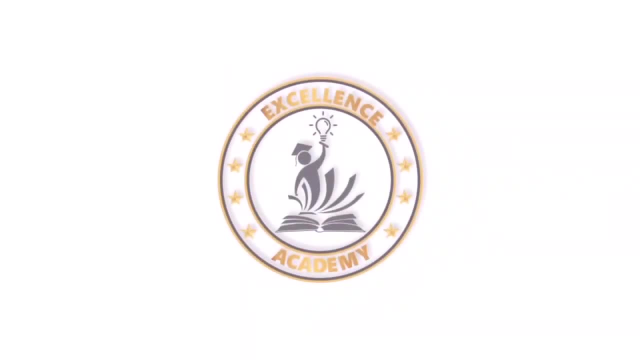 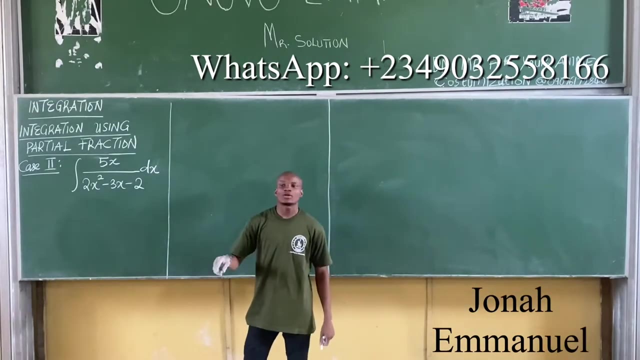 Let's look at case 2 of integration using partial fraction. So you said, for case 2 is when the degree of the numerator is lesser than the degree of denominator. You can see degree here is 1, degree here is 2. So degree of numerator is lesser than that of denominator. 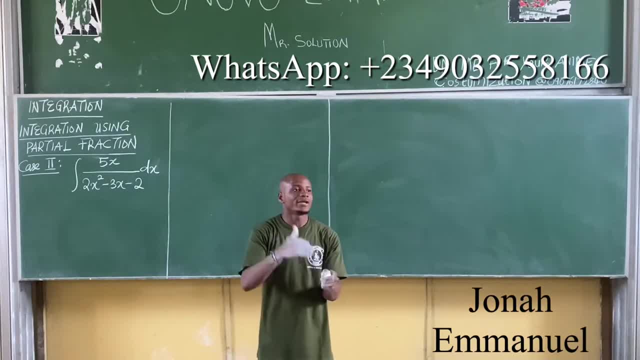 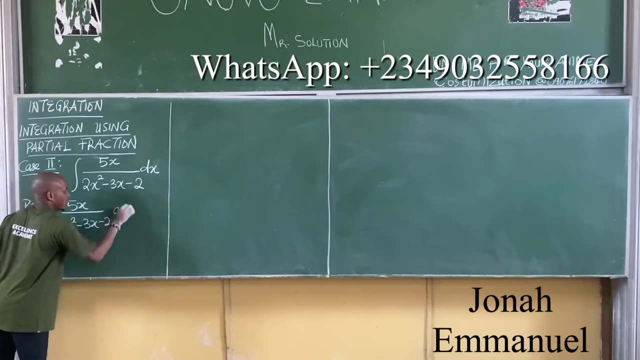 What do you do here? You resolve this into partial fraction, then integrate through How. So your first task here is: pick 5x all over, 2x square minus 3x minus 2, and resolve into partial fraction, Alright. So remember to do partial fraction. I will leave a link to partial fraction in the description of this video. 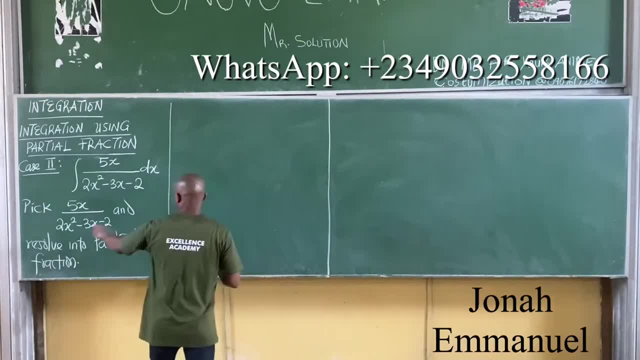 Right, So let's get this one done. So, for partial fraction, our first task is to take this one from your denominator, which is 2x square minus 3x minus 2. Resolve this math, Of course. So this one here is quadratic. If I resolve this, it gives you what there. 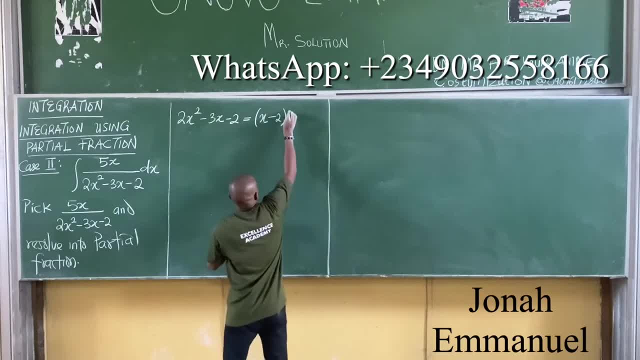 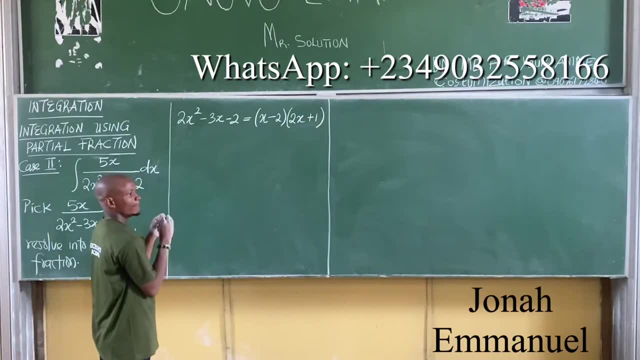 x. what? x minus 2.. x minus 2.. And what do you get there? 2x plus 1.. 2x plus 1.. So I have this. My next task now will be to get the form of the partial fraction. Remember how we do form. 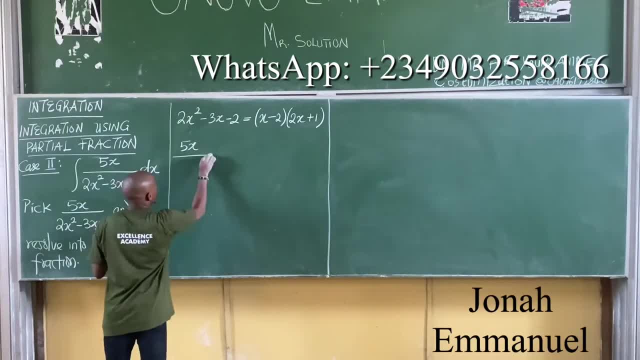 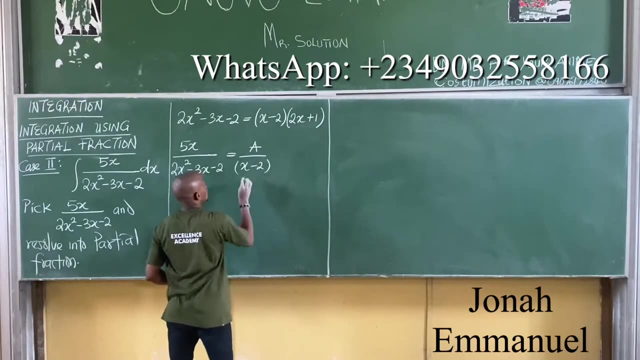 So for this one it becomes what? there? 5x all over 2x square minus 3x minus 2 is equal to a over m, is that right? Yes, So a all over x minus 2 plus b. into what there? 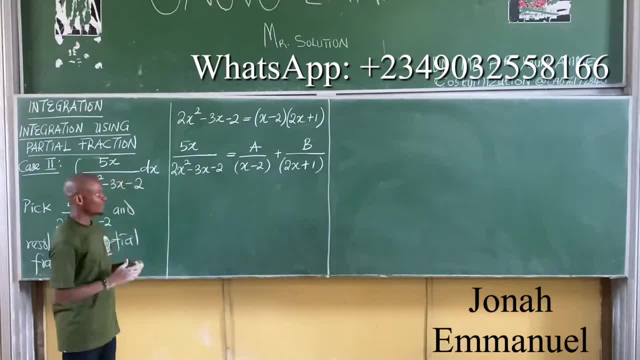 2x plus 1.. 2x plus 1.. Right, So I have this one here. Now it depends on the method of partial fraction you want to use. Of course, for this one here, I will have to combine these two. 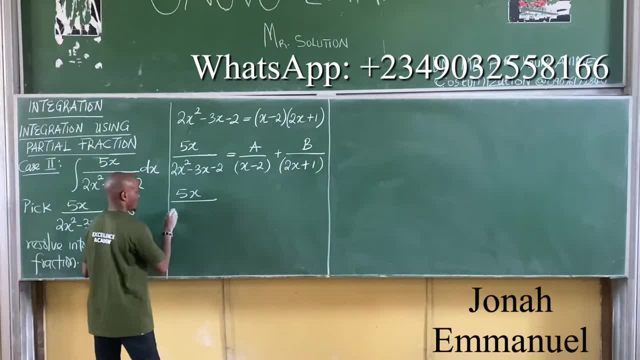 So I will have that 5x all over, 2x square minus 3x minus 2.. x minus 2 is equal to: If I'm combining this, this goes with this as a set. It becomes a into 2x plus 1 plus. this goes with this, b into x minus 2.. 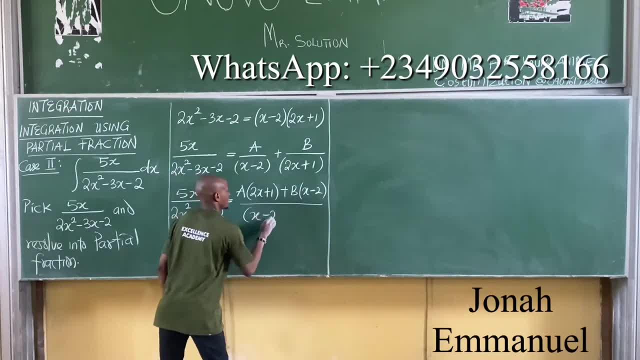 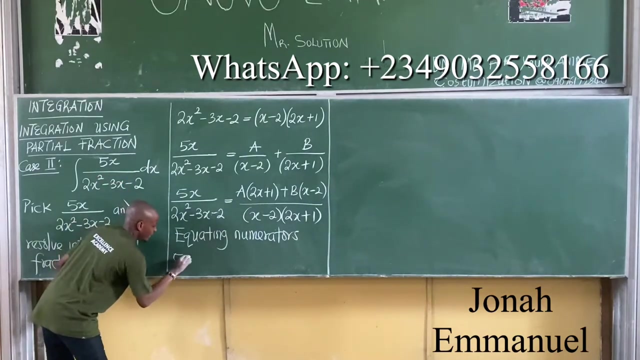 Then combine these two. That gives you x minus 2 into 2x plus 1.. So I have this. My next task now will be equating numerators. Equating numerators: What do I got here? I have that 5x is equal to a into 2x plus 1, plus b into x minus 2.. 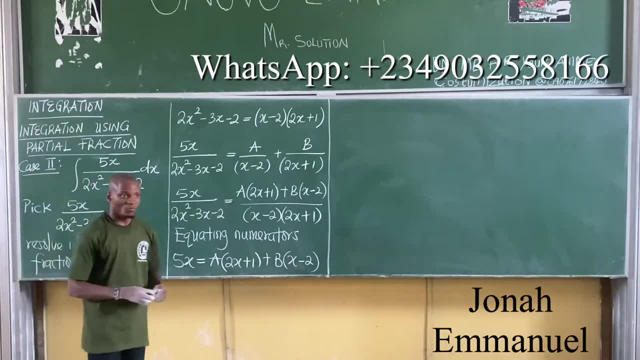 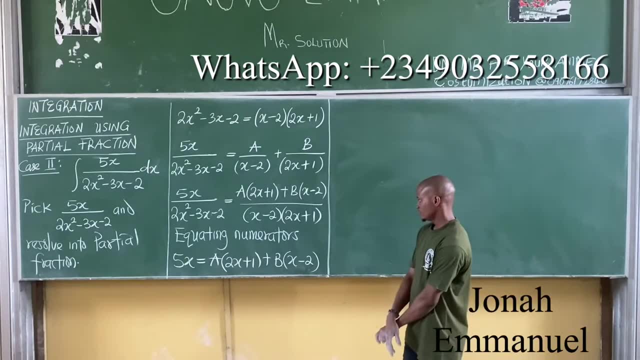 So I have this case here. Which one to do this here? How far off? Which one? 3. If I'm trying to compare the coefficient or Which one to do this here, You can use comparing coefficient now. but Heteroooh is easier, right. 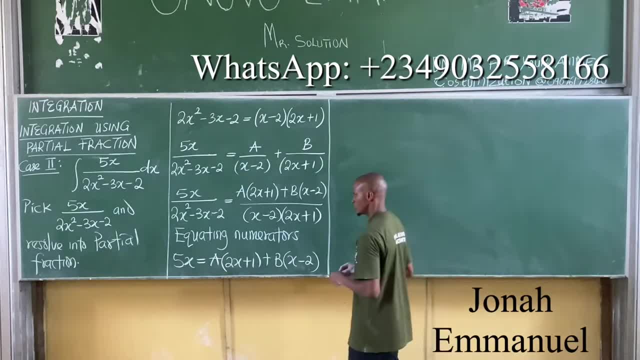 You can use Heteroooh and you just bathtub right here, So let's use Heteroooh method. You can use your normal comparing coefficient. Yes, Let's use Heteroooh To stage time using Heteroooh. 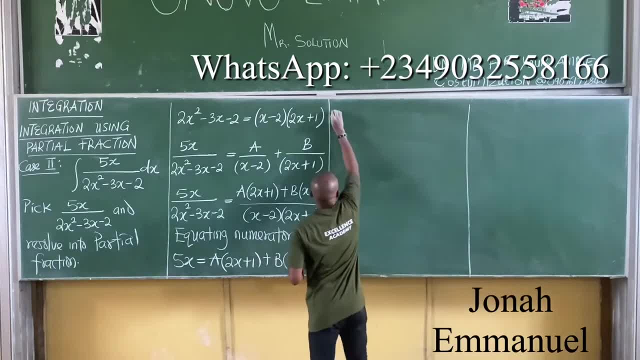 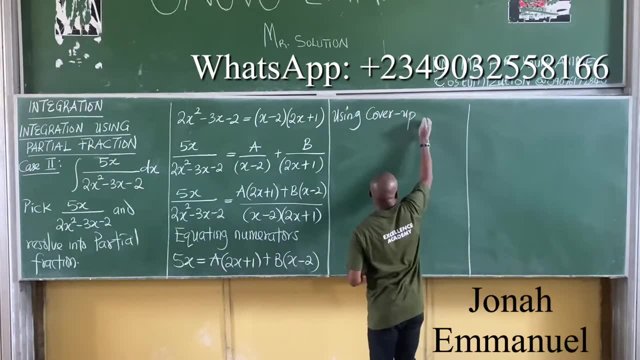 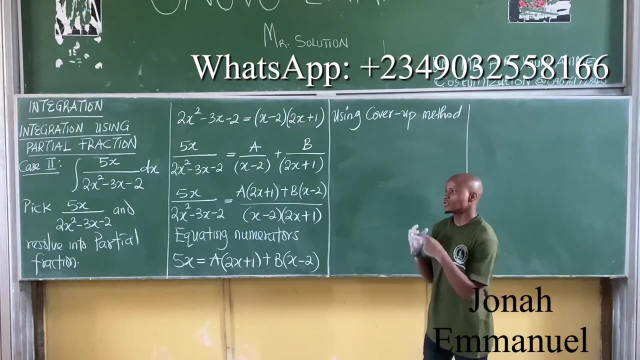 You will give me this object So You can see. Using Kovarov's method. we said the idea of Kovarov is just simple. Watch through this stuff very well. You see a kind of term that you can use to make one of the variables zero. 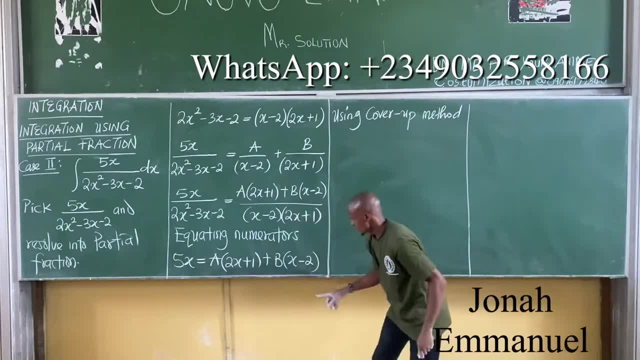 That's the idea behind Kovarov. If I look at this here, this is b multiplied by this. Let's assume I want to make this one zero. What do I do? I equate this term to zero. So I will say that x minus 2 is equal to zero. 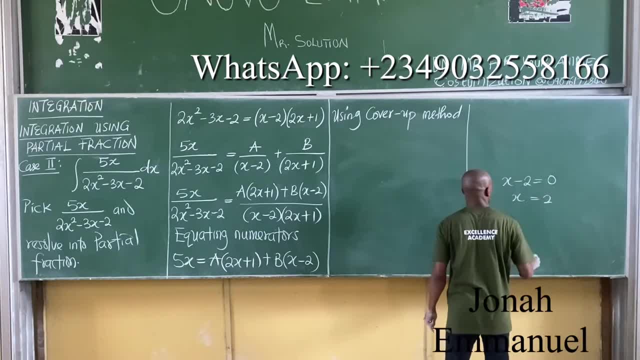 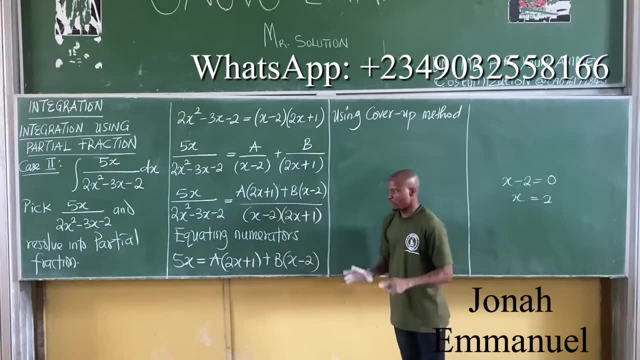 From here this man comes. here x is equal to 2.. That means if I put x as 2 into this equation here, this man will be zero and b will go. So from Kovarov I'll say: let's x be equal to 2.. 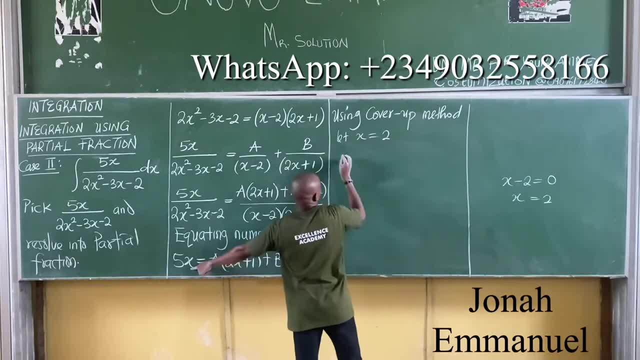 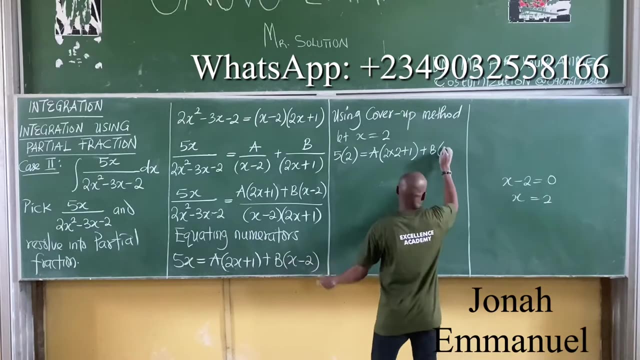 So this now becomes: if I put x as 2 into this, this becomes 5 times 2, is equal to a. A into 2 times 2,, of course, plus 1, plus b into 2 minus 2.. 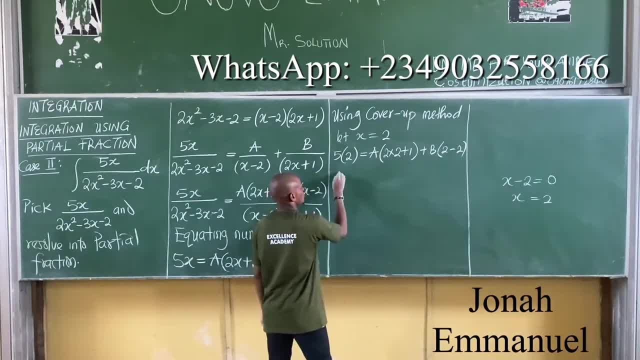 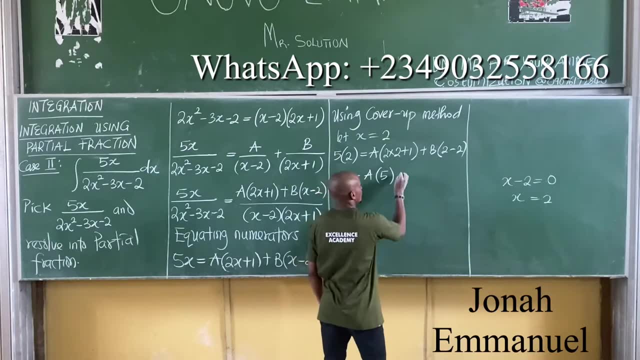 So I have this. What is it that I have? 5 times 2 is 10, is equal to a. into 2 times 2 is 4, plus 1.. That's 5 plus b into 2 minus 2 is zero. 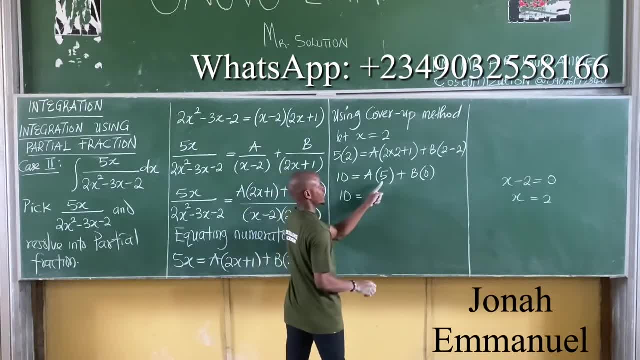 From here I can see that 10 is equal to this and this 5 a b times zero is zero star. I can simply get a here. Divide that by 5.. Divide that by 5.. This counts as this. 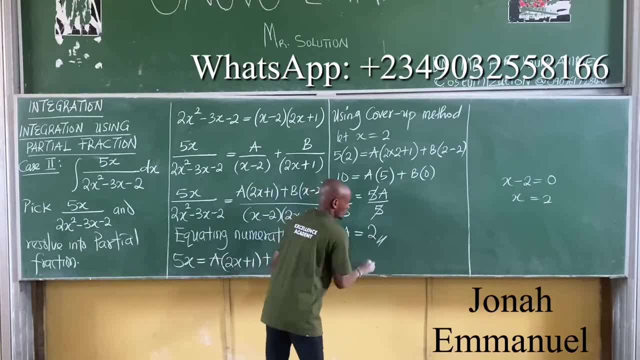 So a is equal to 10 over 5, this one there. So Kovarov is short. You see also very fast. So a is 2.. Let's see if Kovarov can eliminate this one here So we can get b. 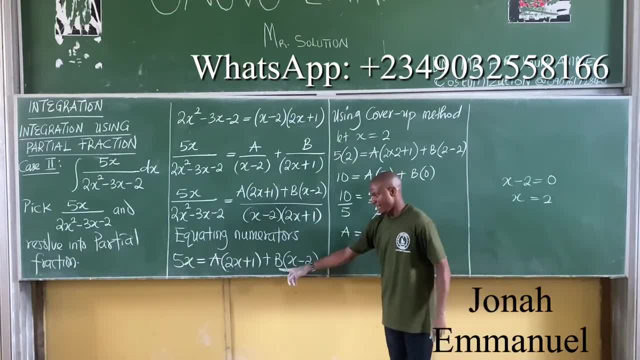 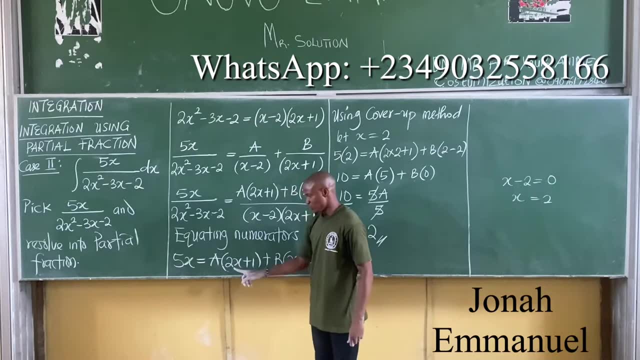 Look at this: If we eliminate b here, we equate this to zero. If we eliminate a, the same thing. equate this to zero. So equate 2x plus 1 to zero. I'll have that 2x plus 1 is equal to zero. 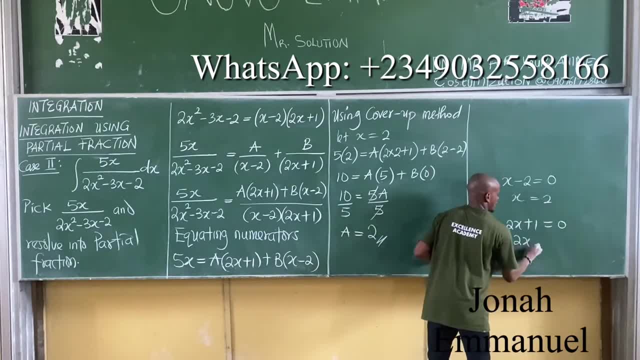 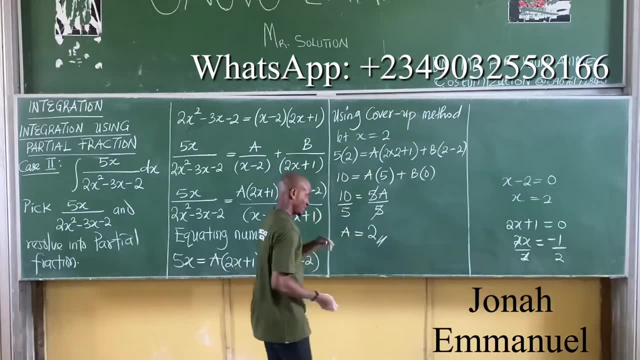 Get x here, Move this one over here. 2x is equal to minus 1.. Divide by 2, divide by 2.. So if I put x as 1 over 2 into this equation, it will eliminate it And give me value for b. 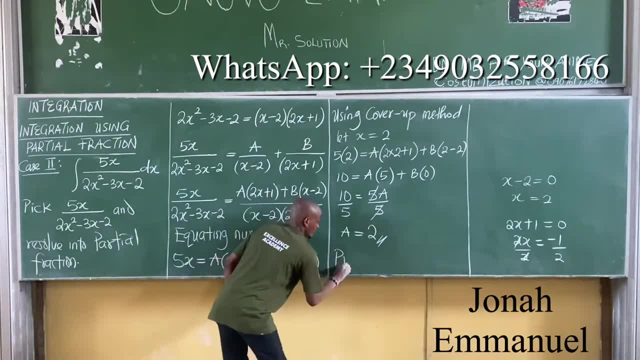 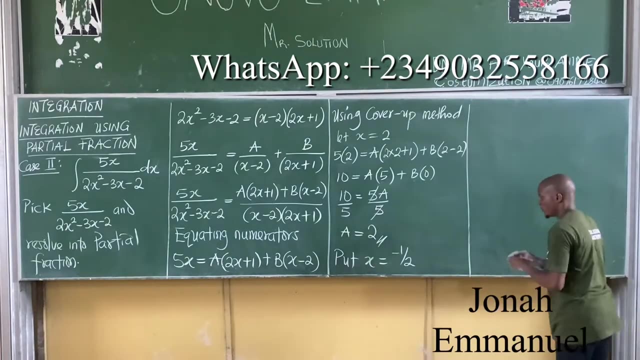 So let's put x as so, put x. put x as equal to minus 1 over 2 into this equation. So that gives you 5 into x minus 1 over 2.. So that gives you 5 into x minus 1 over 2 is equal to. 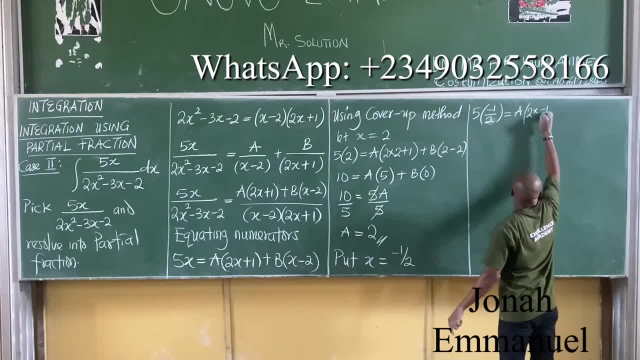 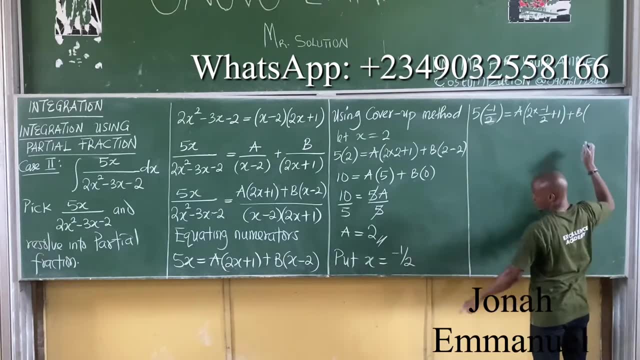 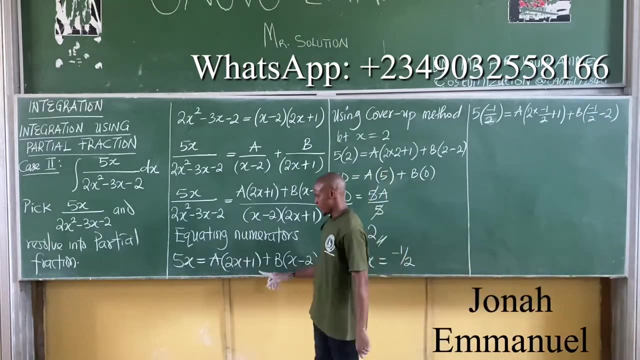 A into 2 times minus 1 over 2 plus 1 plus b into x minus 1 over 2 minus 2.. Let's put x as minus 1 over 2 here. Same thing here. Same thing here. This now gives you minus 5 over 2.. 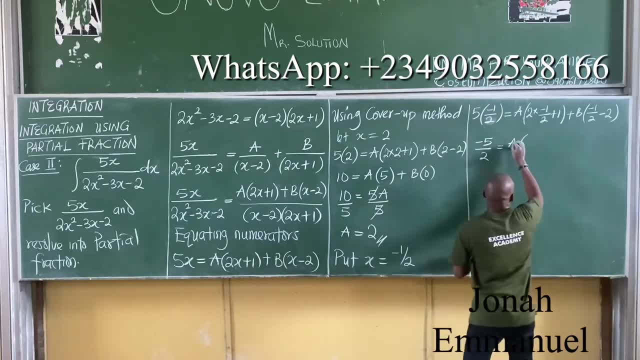 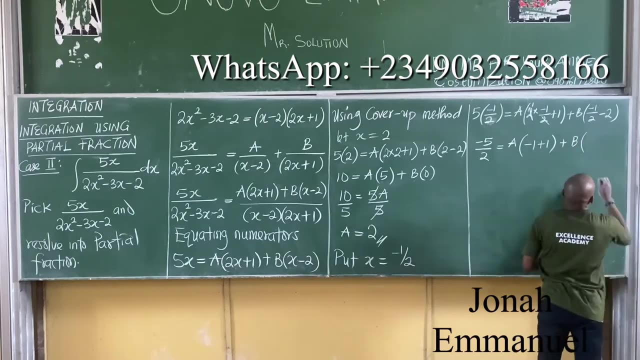 This one is equal to a into from here. this cancels. this is off. It becomes 1.. 1 times minus 1 is minus 1 plus 1 plus b into. what do I have here? This is minus 1 minus 5 over 2.. 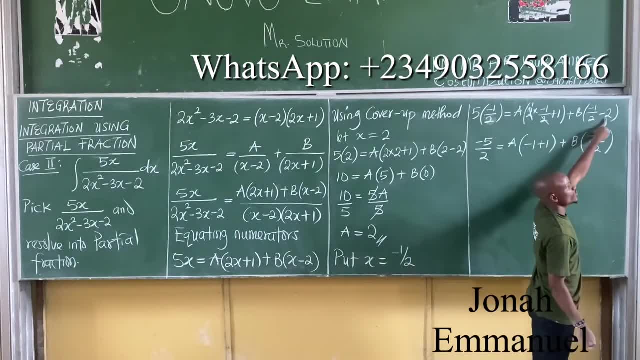 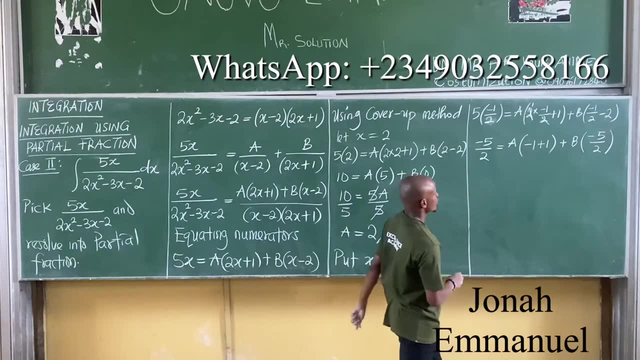 The surface. I've said your shortcut is just to be 2 times 2 is 4.. Minus 1 minus 4 is 2 minus 5 over 2.. Like a shortcut way of simplifying this. So this is what I'm having. 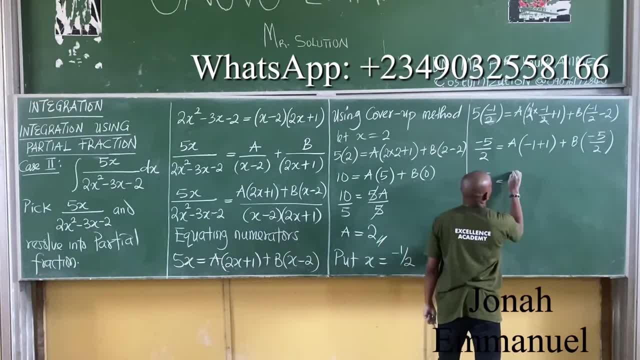 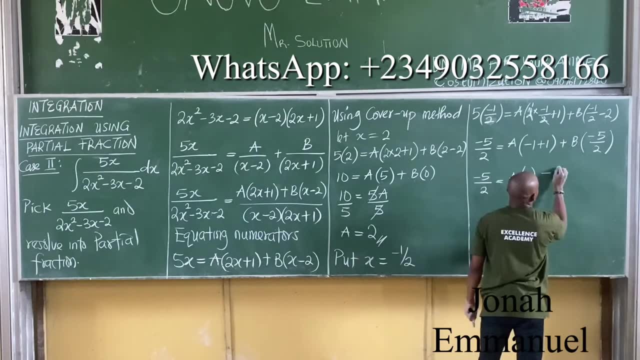 Minus 5 over 2.. Minus 5 over 2 is equal to a into minus 1 plus 1. That's zero Plus times minus Minus 5 times b, 5b all over 2.. So this is off. 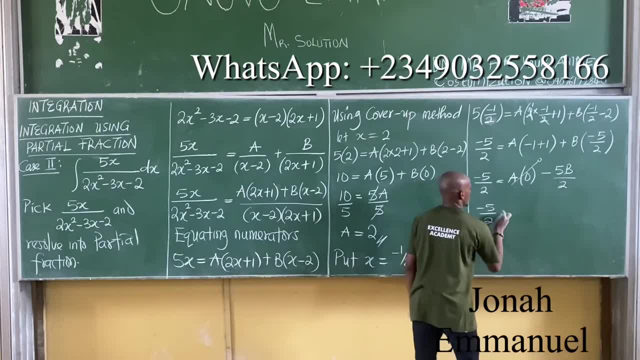 Zero, And that is minus 5 over 2 being equal to minus 5b all over 2.. Just by a mathematical sense, Minus times minus, You might have the same term on both sides, So 5. If they are multiplying they can cancel out. 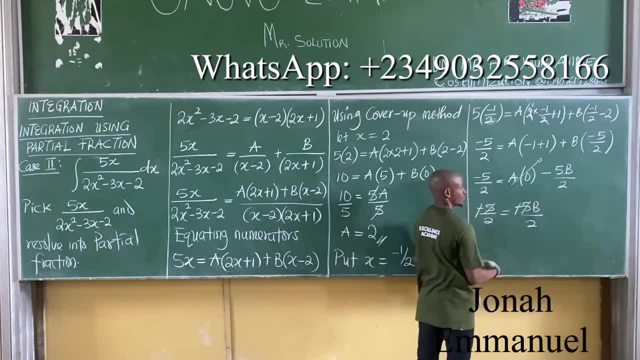 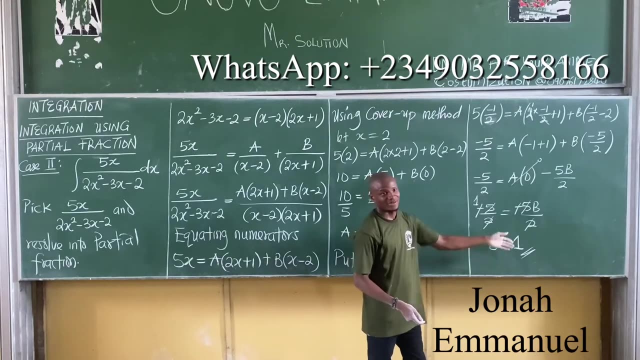 So minus cancels, minus out, 5 cancels, 5 is off, 2 cancels 2. And that is 1 here. Alright, From here now, b is equal to 1.. So I have this If you want to continue your normal basic maths, right? 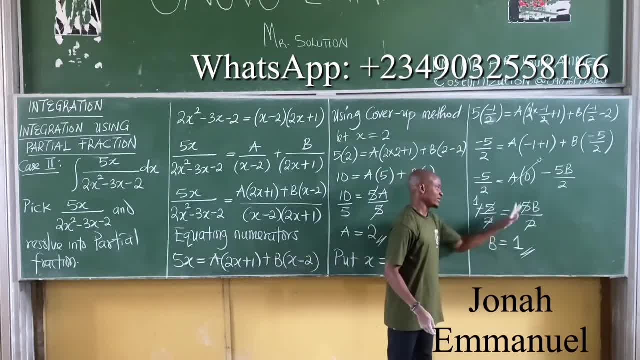 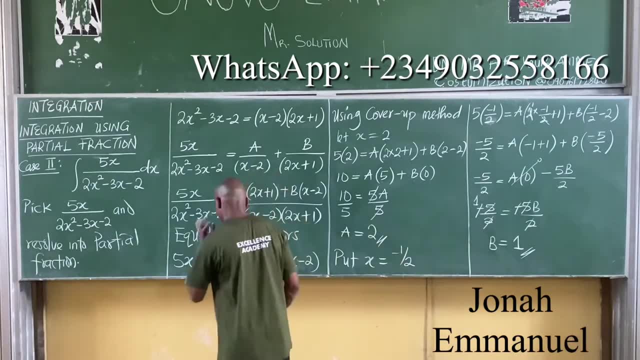 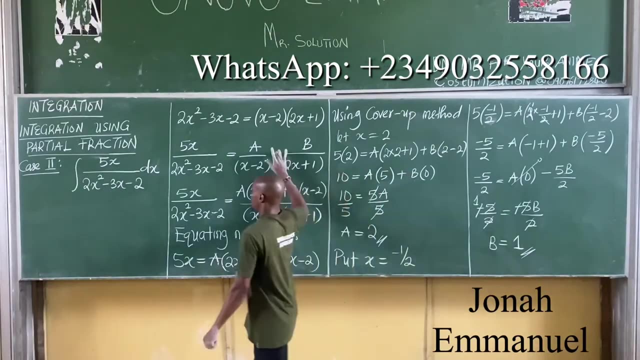 Here I have 1.. But simple concept, The same thing here. It cancels out to give you 1.. So hence, a is 2.. b is 1.. Alright, If I put this 2 value here, I will now have that yx all over 2x squared minus 3x minus. 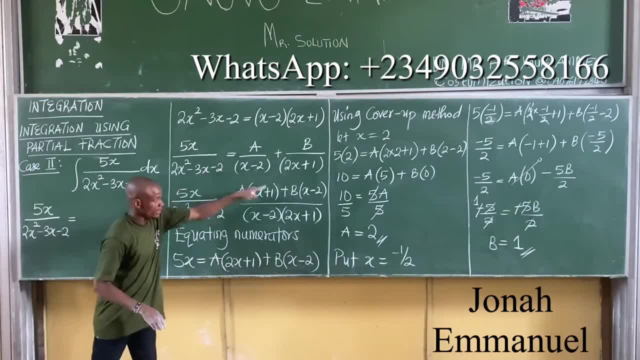 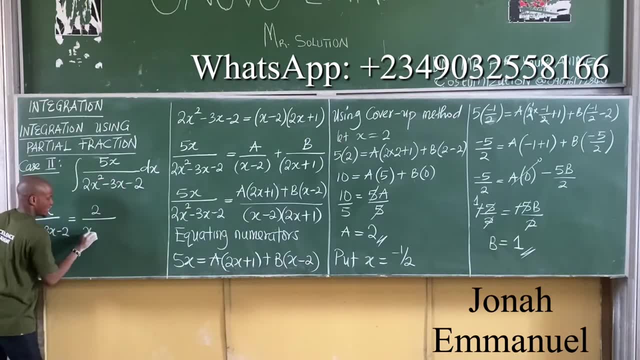 2 is equal to a, a is 2.. So it becomes 2 all over this one here. Alright, x minus 2.. Next up, Plus b becomes plus b is 1.. So it becomes 1 all over 2x plus 1.. 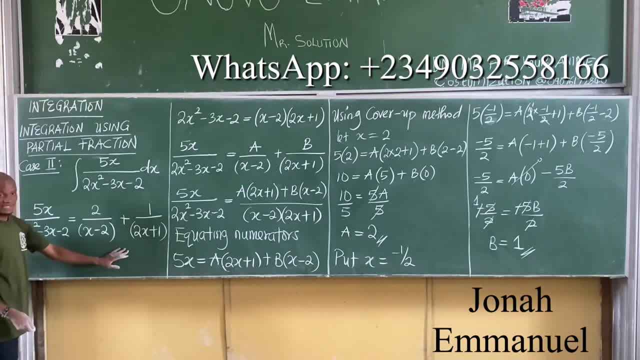 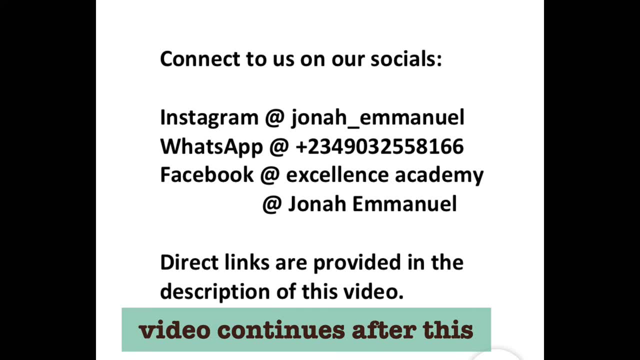 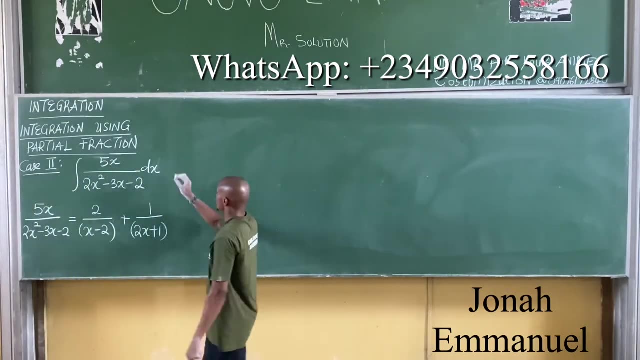 So if I resolve this into partial capture, I will have this Alright. So from this let's integrate 2.. So hence it means that the integral of 5x all over 2x squared minus 3x, minus 2x, will. 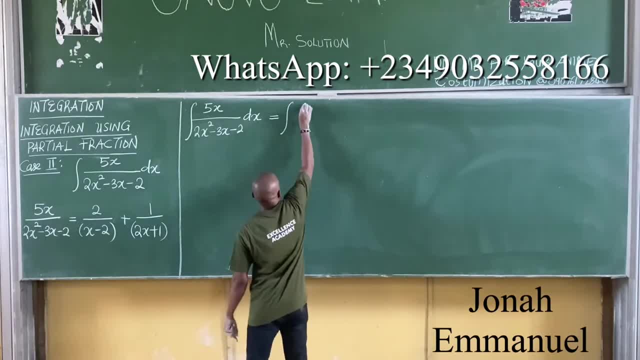 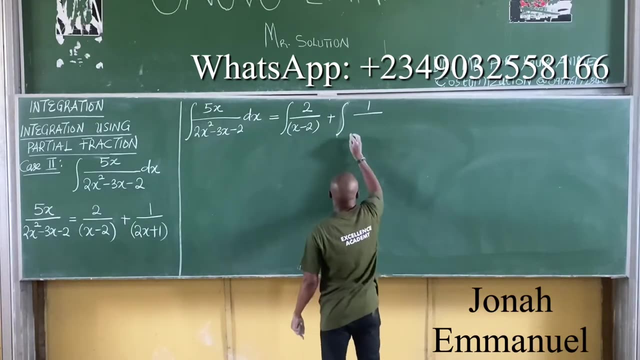 be equal to the integral of 2 all over x minus 2.. Plus the integral of 1 all over 2x plus 1.. Of course, each of them is dx. So how is this equal to say? take constant n outside, to the outside. 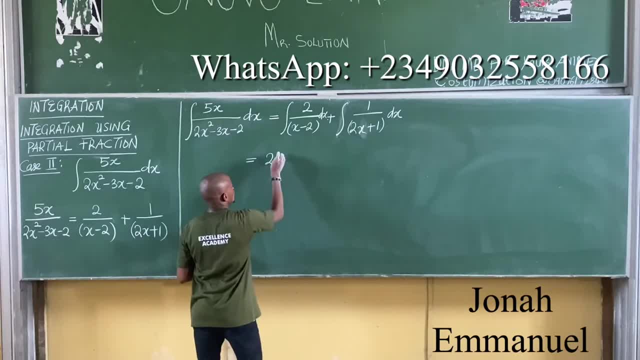 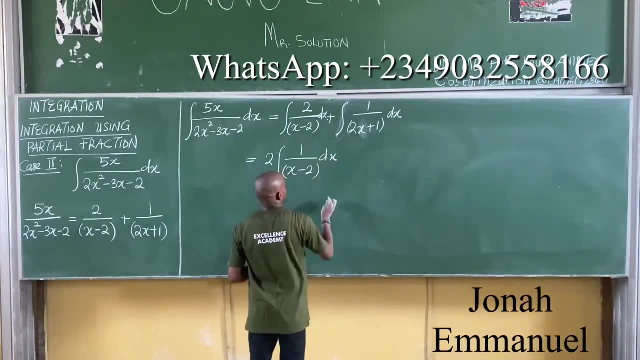 Constant n is 2.. It becomes 2 integral of 1 all over x minus 2 dx plus. having at least 2 here is not a constant. Alright, It gives you integral 1 all over 2x plus 1 dx. 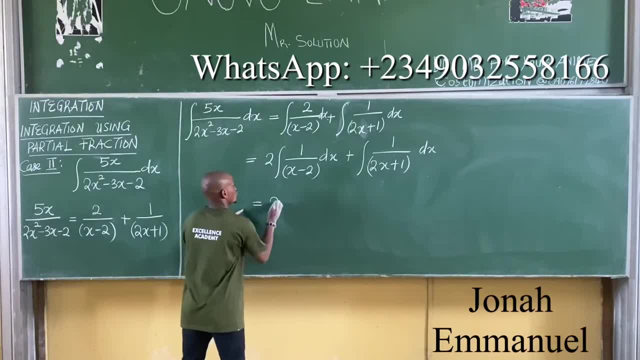 We know what is for this. here That's equal to 2.. This gives you what there? x minus 2 plus This one gives you length Of them. here it's still linear, It's 2.1.. So it's still linear. 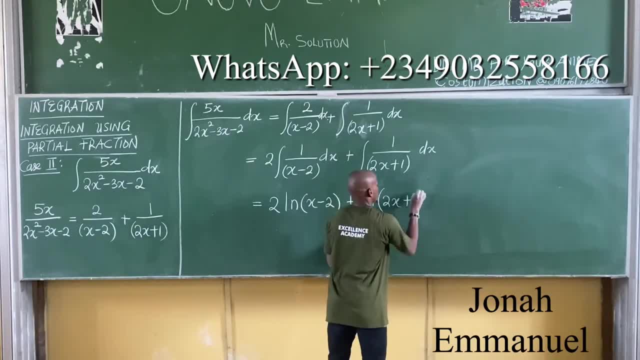 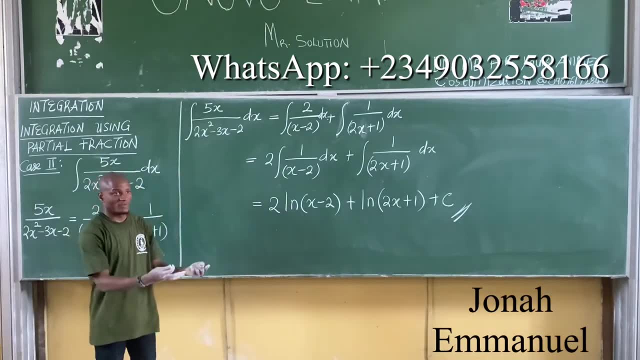 So it gives you what there? 2x plus 1.. Next, one Plus c. This becomes the answer to this equation. So the task is simple: Resolve this to partial capture, Then it will be true. You have this. That's how you solve this question. Thank you.